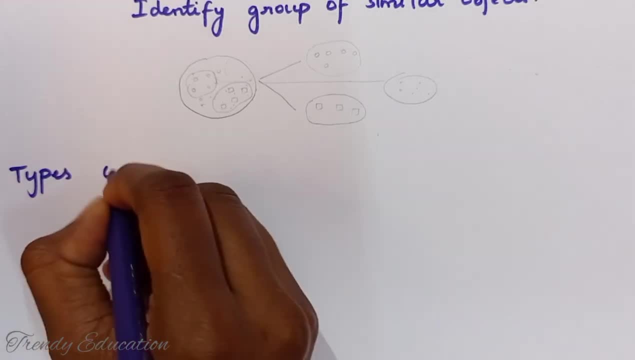 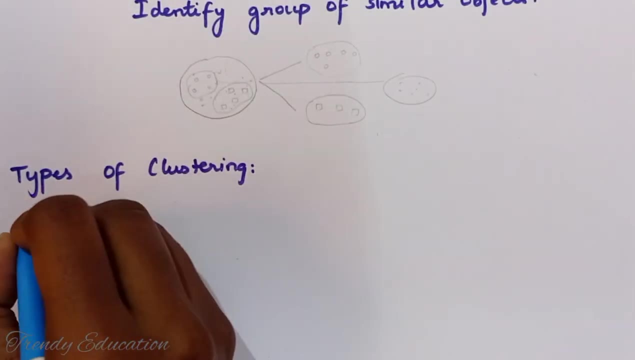 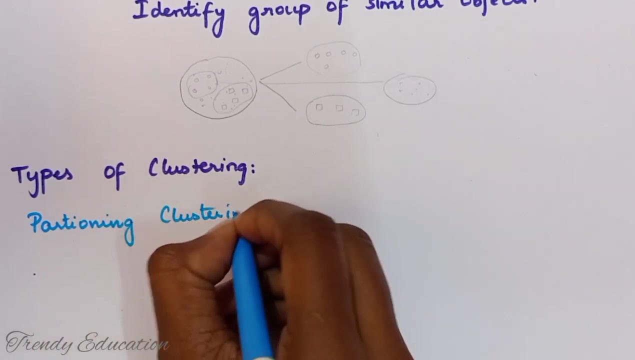 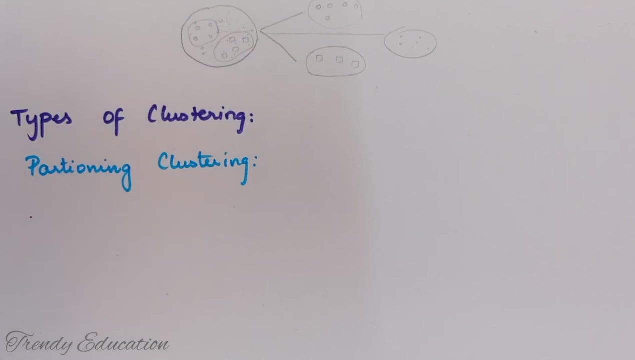 first clustering we are going to see is partitioning. so what is partitioning clustering? and this clustering is a very basic clustering in types of clustering and in this what we are going to do is we are going to give a set of data that like this, and we are going to get 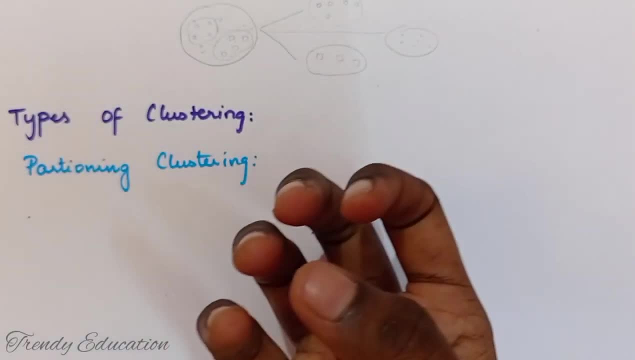 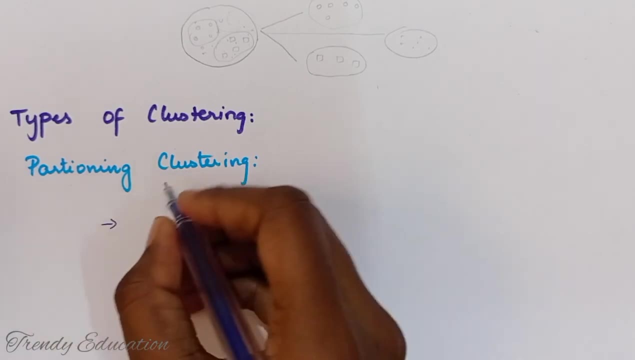 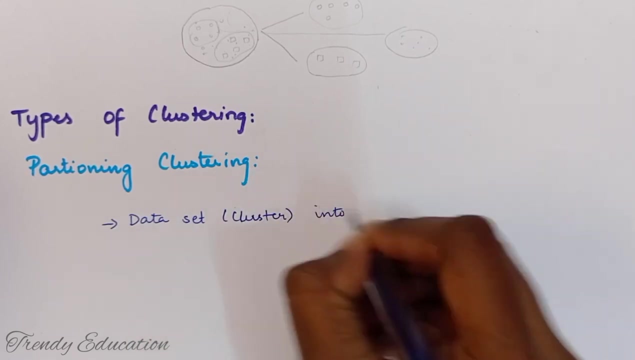 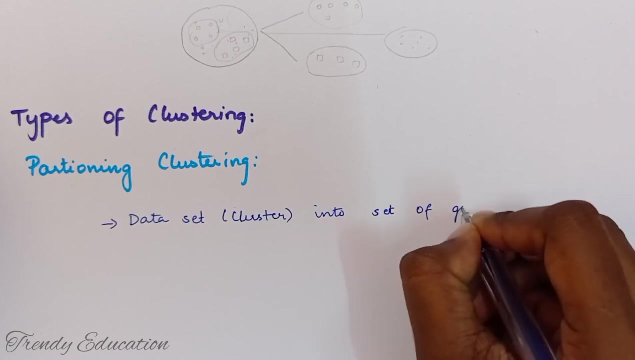 number of outputs, that is, the groups are called as clusters. so what we are going to do is we are going to, we are going to cluster the data set- sorry, cluster into set of groups, cluster data sets into set of groups. and then what the major step in the partitioning clustering is? 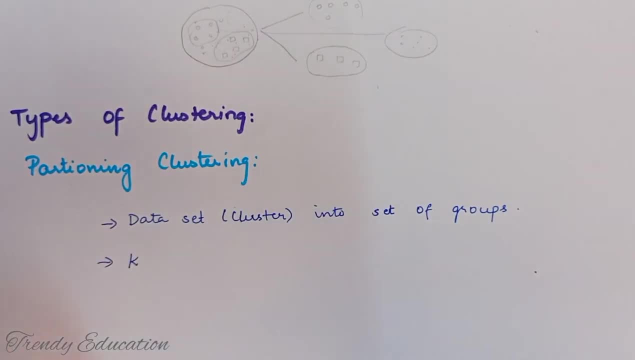 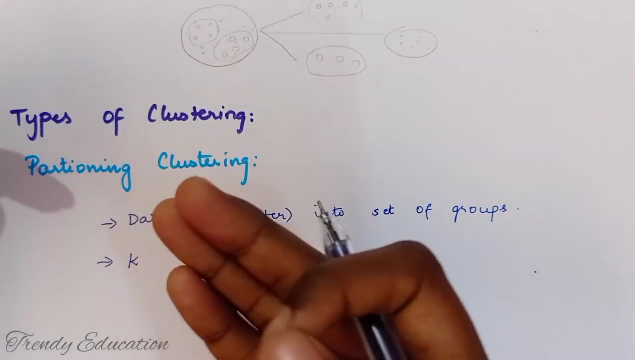 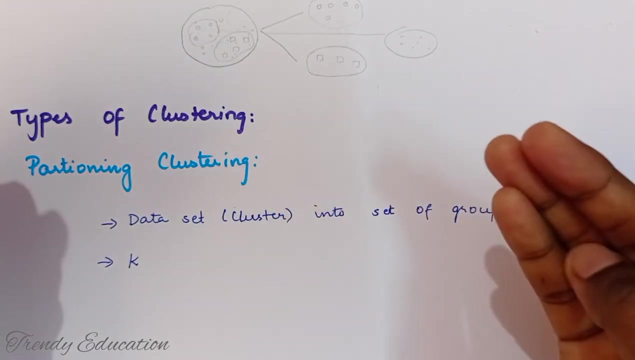 we are having something called as k. so what is this? k is called as the cluster, the number of the cluster. so we have to pre-define, that is, pre-specify, the number of the clusters. that is, we have to pre-specify the k value before the data is going to process. that is, the data is. 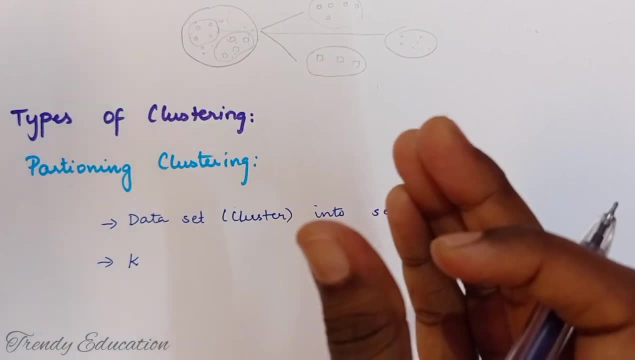 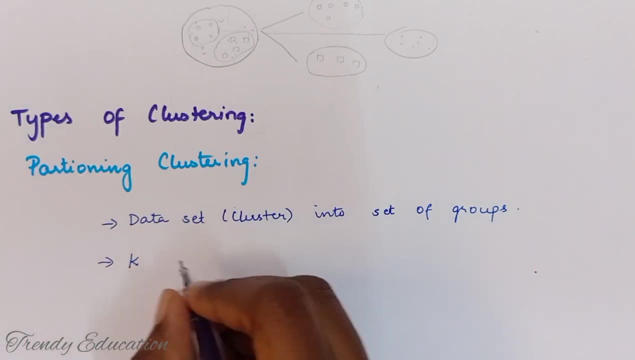 going to cluster, we have to enter this value before clustering. so this is why the k k value is nothing but so when i'm giving three, that is the k value equal to three, then the data object, that is, the total data objects, is classified into three clusters. 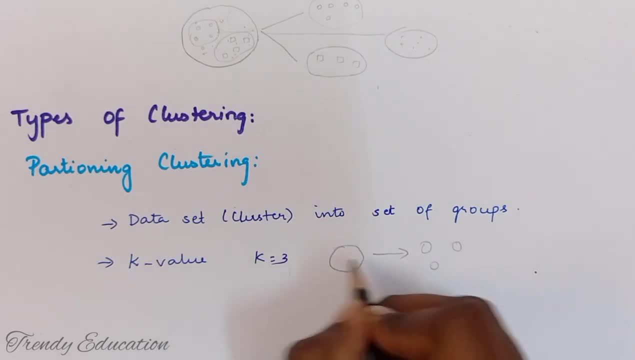 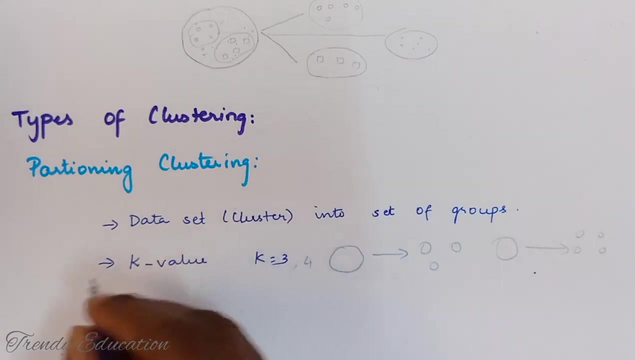 but when i give four here, but then it is class, that is cluster into four, four groups. so this is what this k value. this partitioning clustering is totally based on centroid based method. so what is centroid based method in the sense here? a centroid, something called a centroid, which is used, so mostly the plus symbol is used. 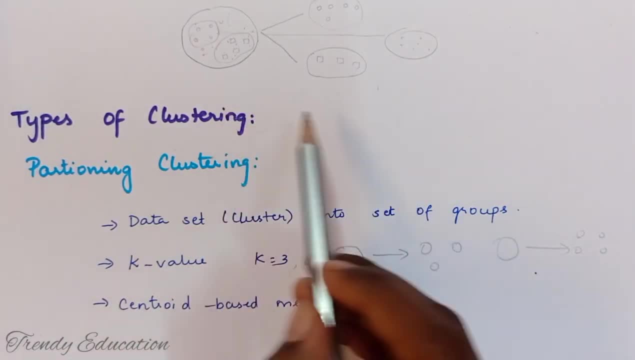 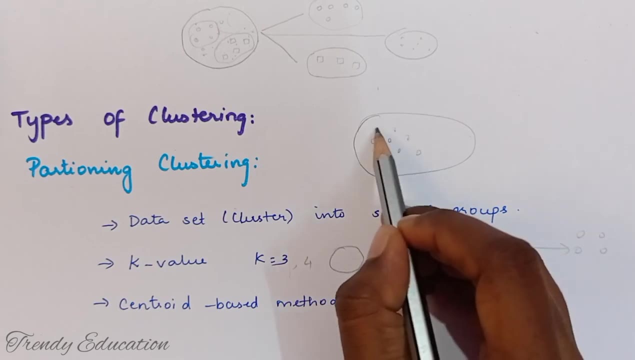 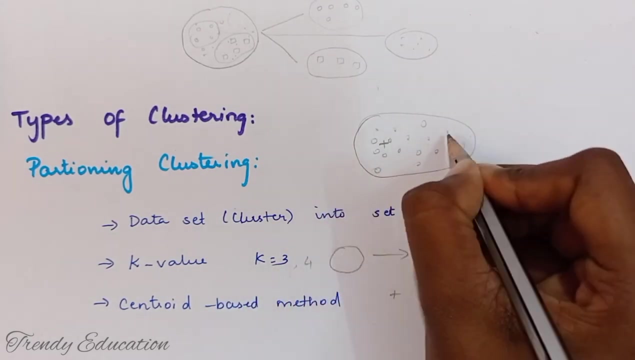 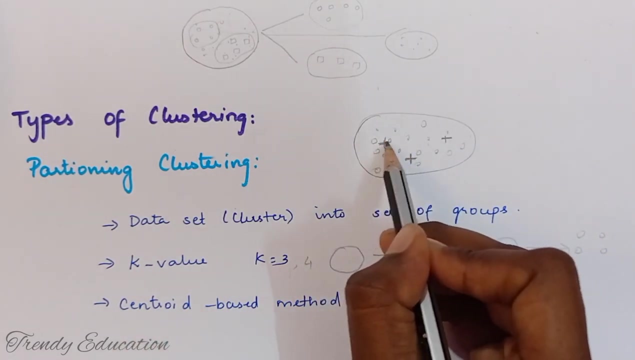 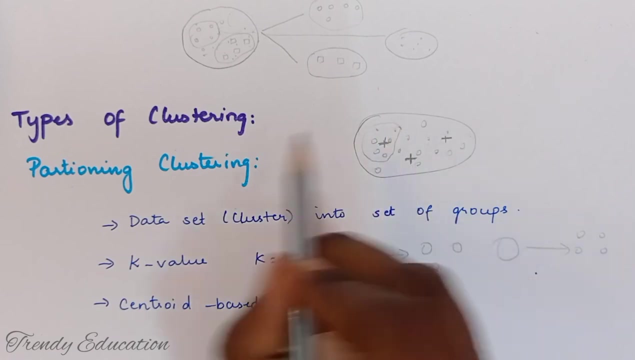 as a centroid. so here what people will do is they will use the plus symbol. i will draw here and i'm giving the k value equal to three, so i'm using three plus symbols. this is centroid, so i'm using the centroid, this is the centroid and the data around the centroid will cluster as a single data set. 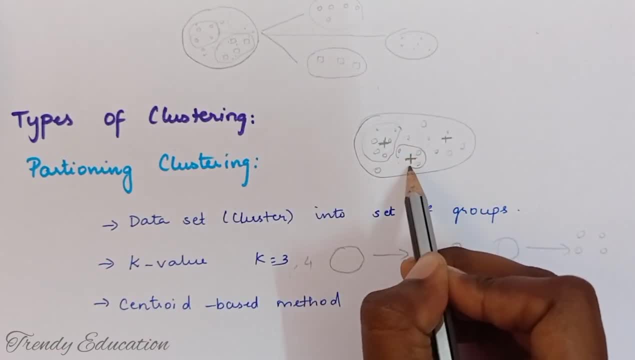 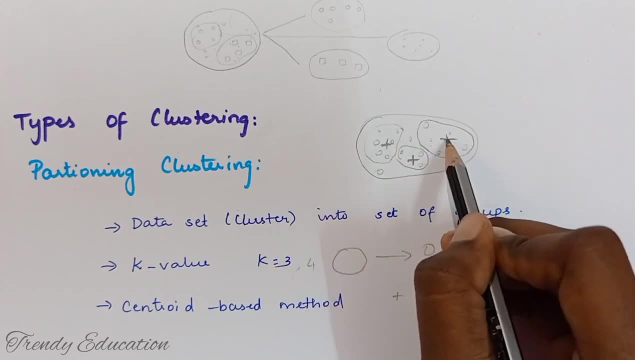 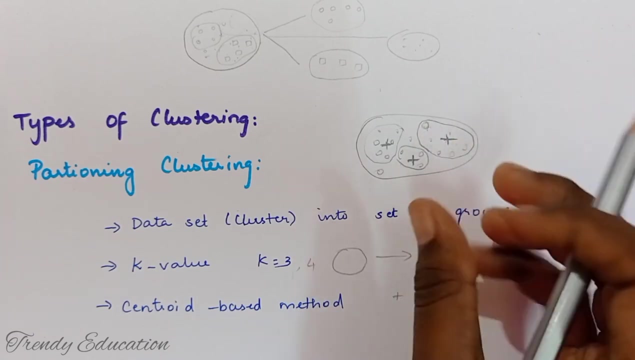 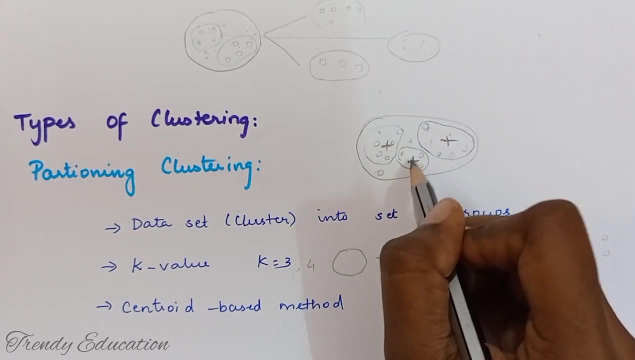 and this is a single say, that is single group and this is a cluster. the distance between the centroid and the data object is measured and the object will cluster into the group in which the distance is very short, so you can easily predict the distance between this. and this is equal, so it can be anything. 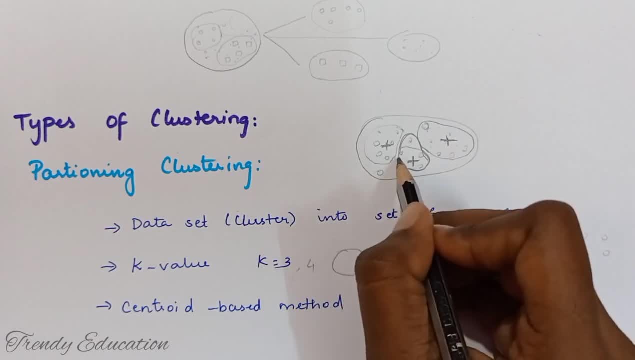 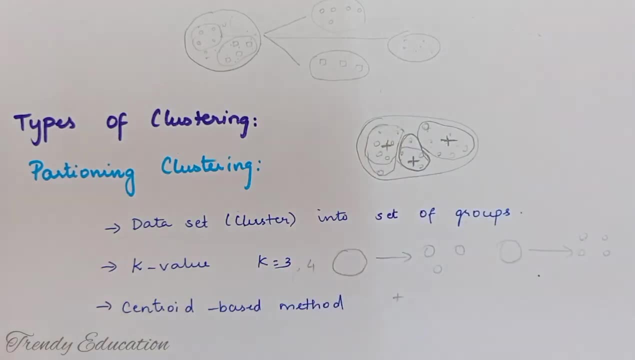 it will get into any group it wants. so the distance between- and this is this- is also merely equal. so i am clustering. this is as a group. so when i am giving k equal to 3, which means there are three centroids, so i'm clustering, it has three groups. 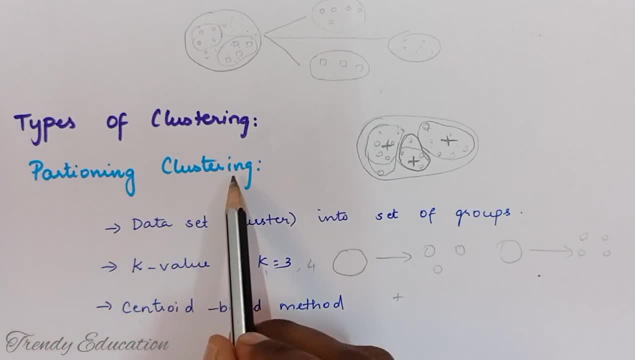 also called as three groups clusters. i hope you understand what is partitioning clustering: the data sets is clustered into the set of groups using the k value, which is called as the centroid based method, and here i already told that we are going to pre specify the number of clusters. so these are the major point. 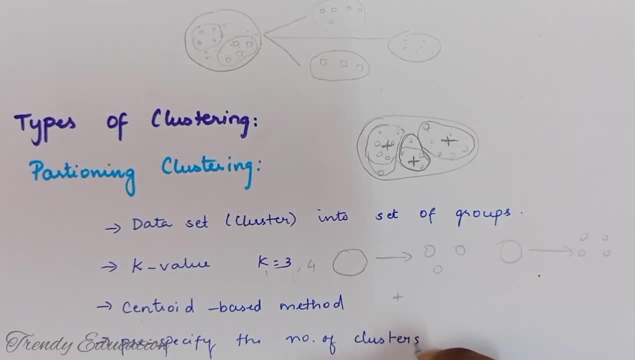 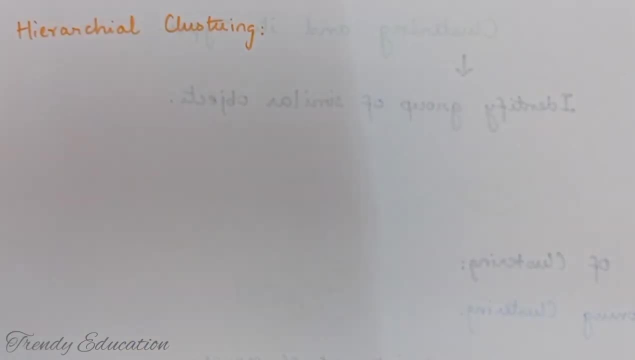 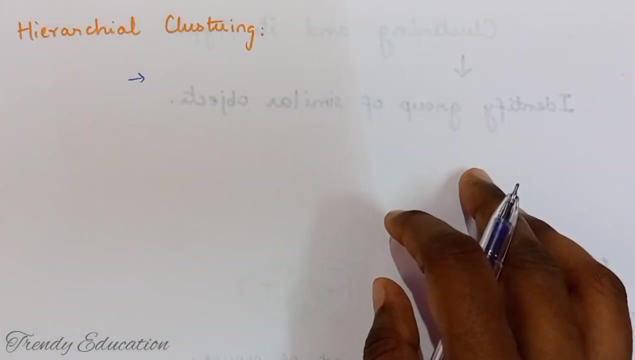 of the partitioning clustering. so let's move on to the hierarchical clustering. and yeah, now coming to the hierarchical clustering, and this is similar to the partitioning clustering and here we are going to set in partitioning clustering. we have to pre-specify the number, but here we are not going to pre-specify the number of the clusters, so no need to pre-specify. 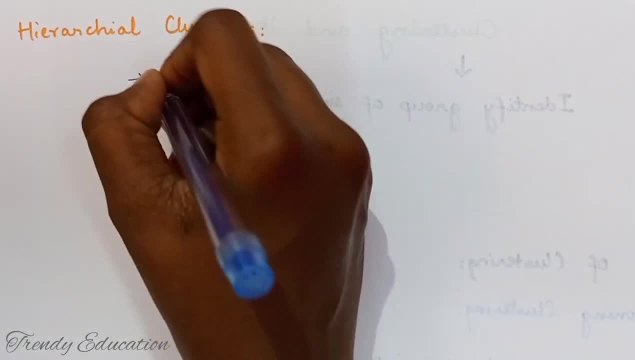 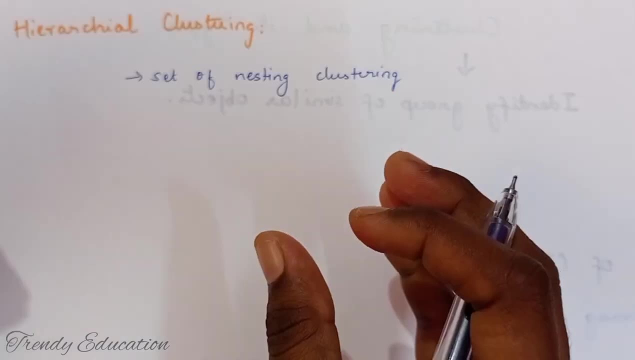 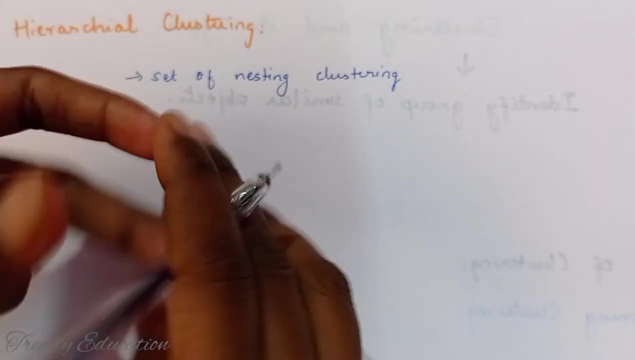 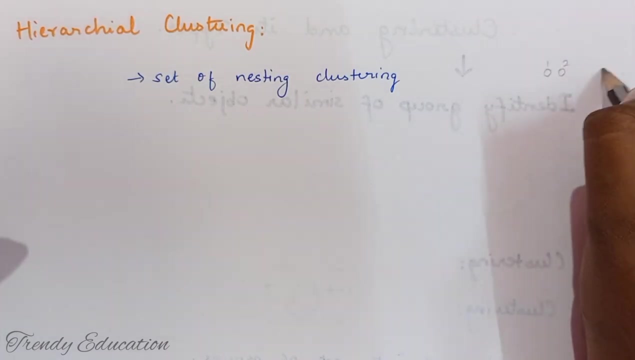 so what we are going to build here is set of nesting clustered. so what is nesting clusters? in the sense a cluster is cluster into another cluster, a cluster which is cluster into another cluster. i'll explain you now. so here you can see there is two objects, and this is one and two. 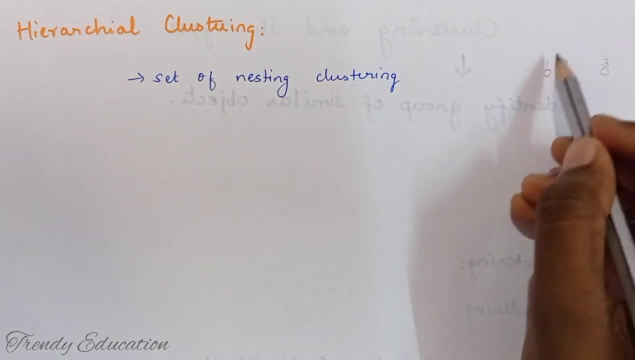 and this is three and this is four. so i am clustering these two as a cluster and again these three as a cluster and again these four as a cluster. you can see that a cluster- one cluster- is clustered into another cluster, and now, when you convert this to a cluster, one is also clustered into another cluster. 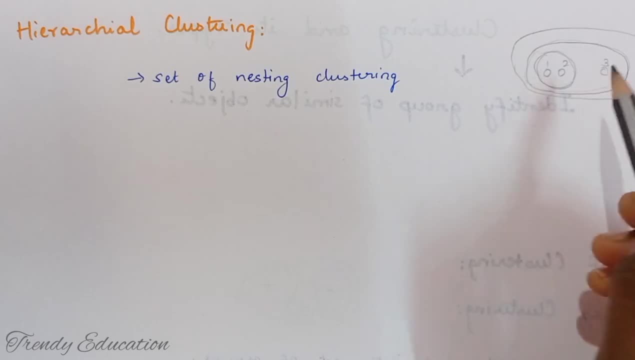 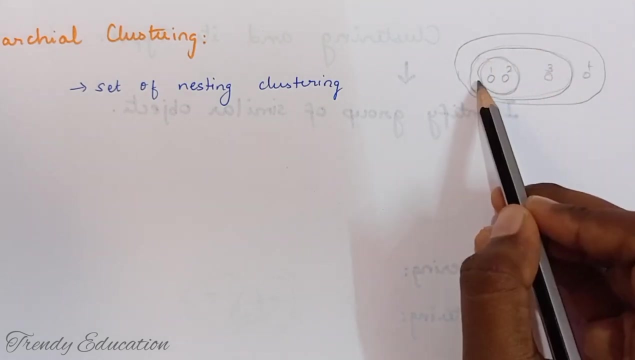 If you are not familiar with neighboring clusters, then you can use this in the future to solve this problem as a Pixel Test. so this is what a nesting cluster. so hope you understand this hierarchical clustering. a cluster is cluster into another cluster and again like this. so this is what hierarchical clustering. 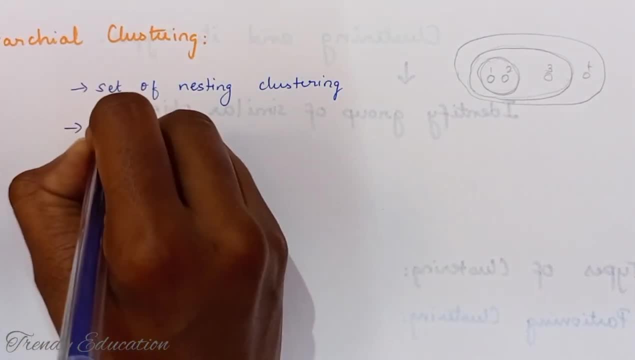 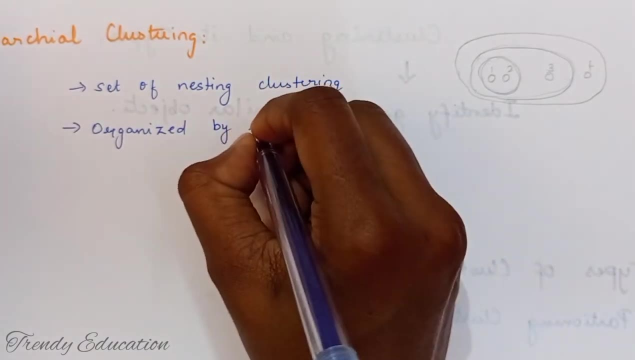 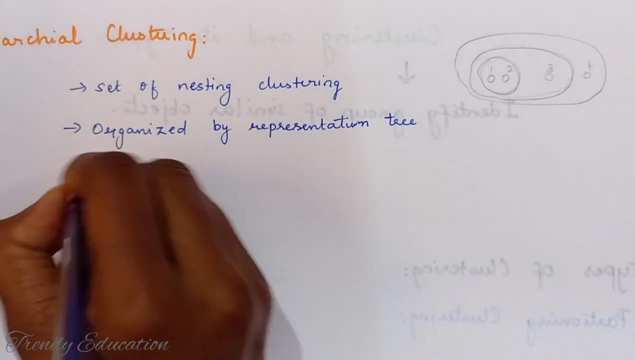 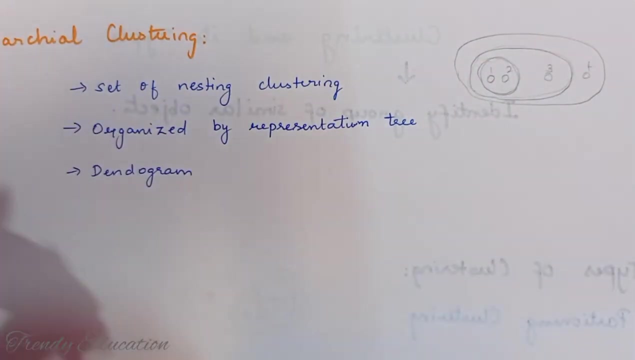 and here it is also organized by tree, organized by, that is, this nesting is also organized by the representation, like representation of tree, which is called as dendogram. we call it as dendogram. so what is dendogram? i'll explain you with this example. now, here one and two are cluster. 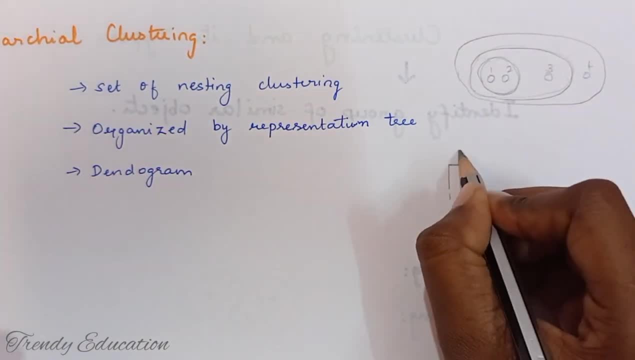 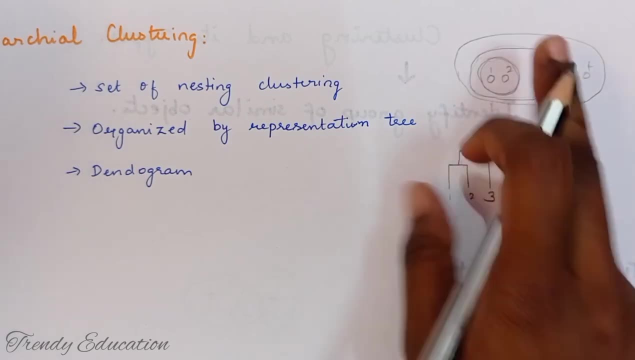 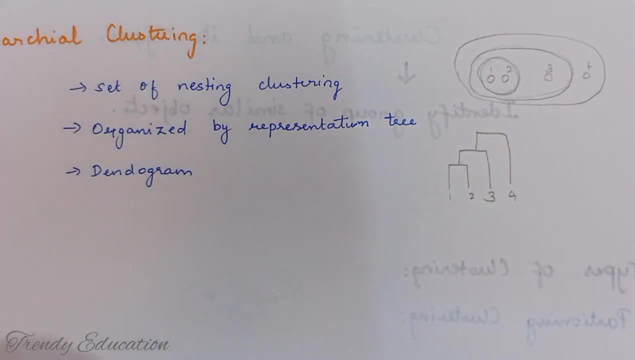 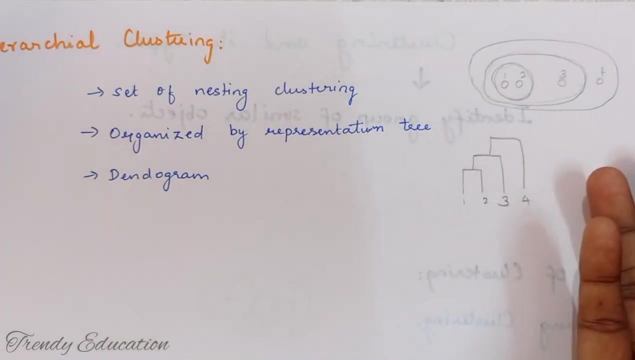 into a cluster: one and two, and again it is cluster with three, and again it is cluster with four. so this is what dendogram and this is what dendogram and this is nesting, that is, nested clusters. hope you understand what is hierarchical clustering and i'll explain you detailly these topics in separate videos, that hierarchical clustering in a separate. 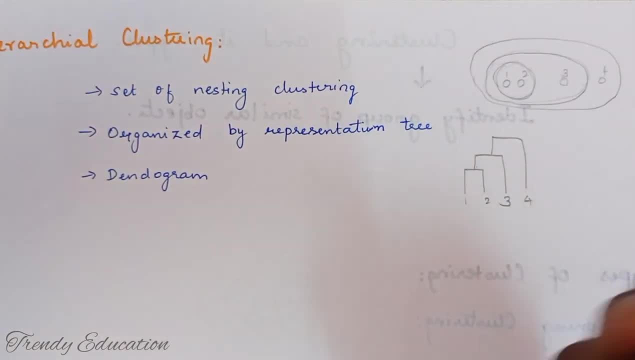 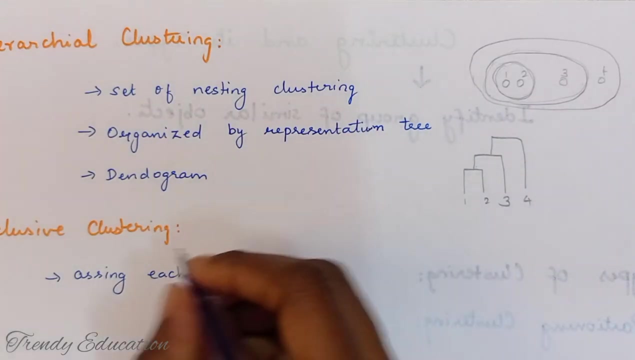 video detailly, but here i'm just giving you introduction about the types of clustering. so let's move on to the next clustering, which is the exclusive clustering. and this clustering is very easy clustering. And here what we are going to do is we are going to assign each object, that is, each object, each and every object- to a set of groups, that is, to a group that is a cluster. 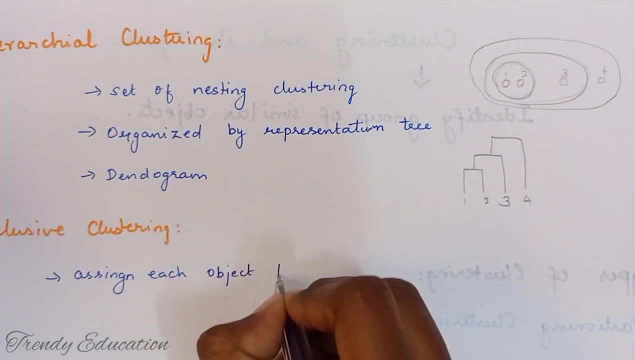 Assign each object to a single group. that is, one object must be present in only one group and not in other groups. One object, that is, objects in this group, must not be available in this group. So this is what: each object to a single group. that is single clustered group and it is also called a non-overlapping clustering. 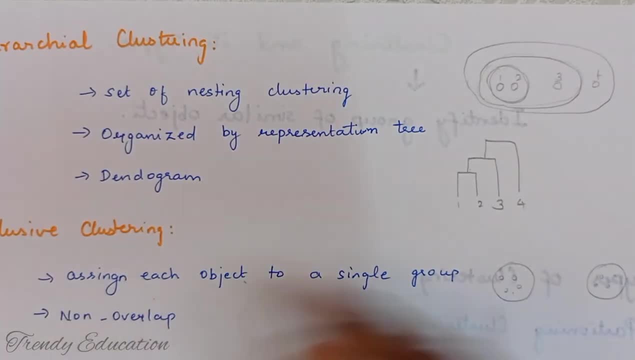 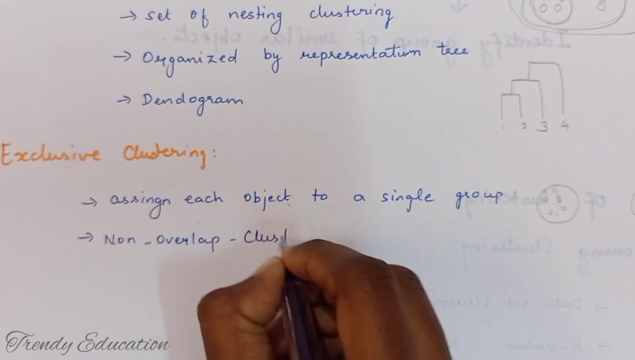 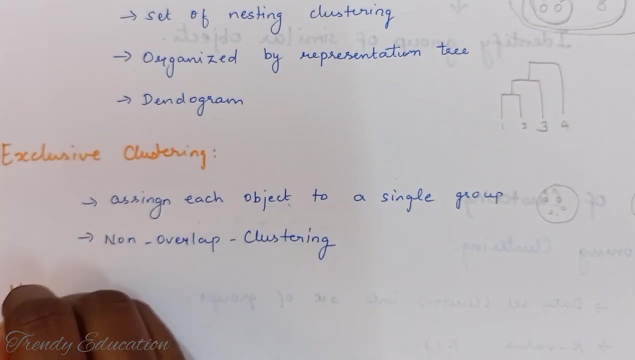 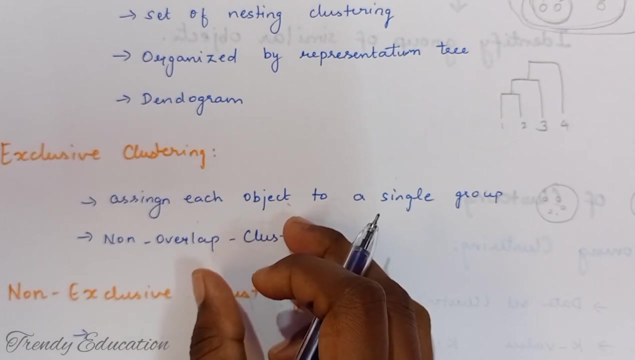 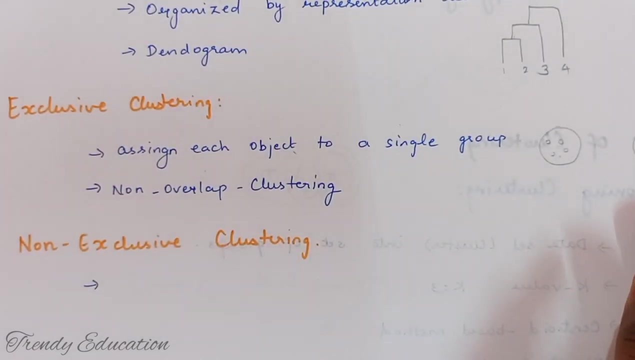 You can see, there is no overlapping between this and this clustering. there is no overlapping. And now moving on, Moving on to the non-exclusive clustering. So what is non-exclusive? in a sense, it is just exactly opposite to this. And here objects can be present more, that is, objects in one group can also be present in another group. 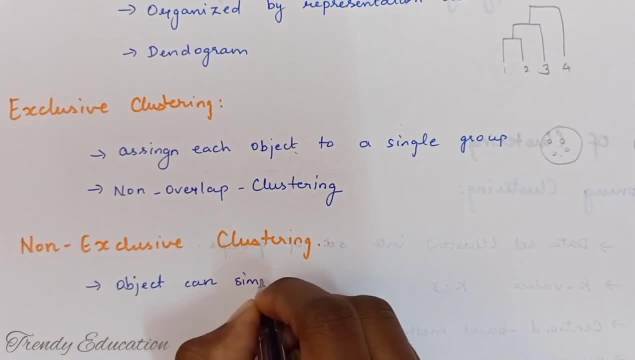 And here objects can be present more, that is, objects in one group can also be present in another group Simultaneously. we can use the word simultaneously. objects can simultaneously belongs to more than one group, One or more than it can, either one or more than one also. 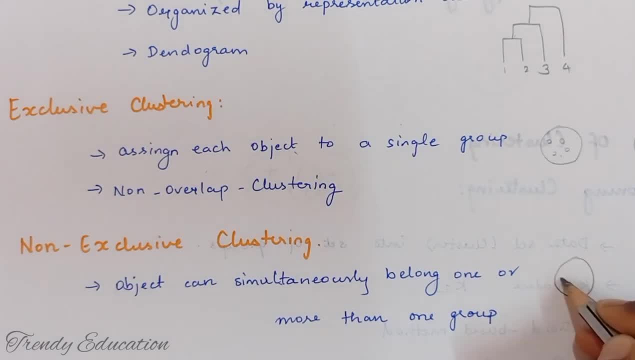 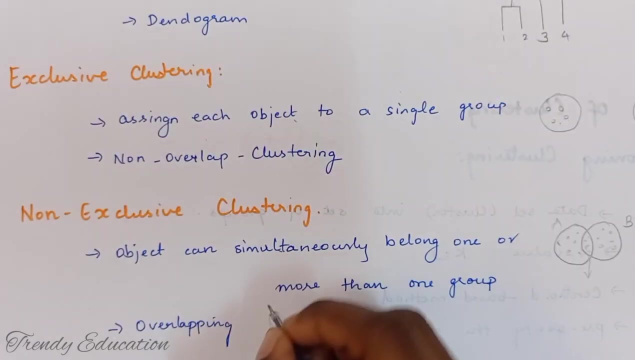 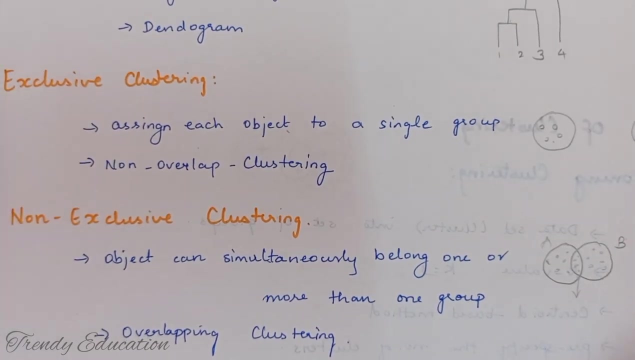 And here what how it is like is: There is some objects in A and there is some objects in B and there are some objects in this common area intersection. So it is also called a overlap, that is, overlapping clustering. And yeah, now move on to the next clustering type. 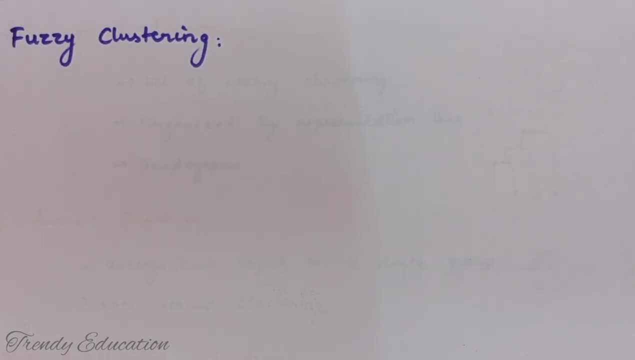 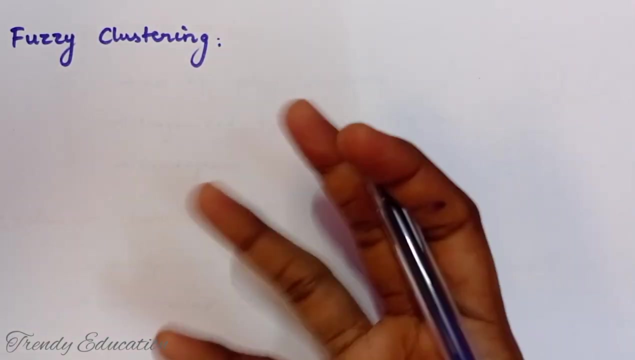 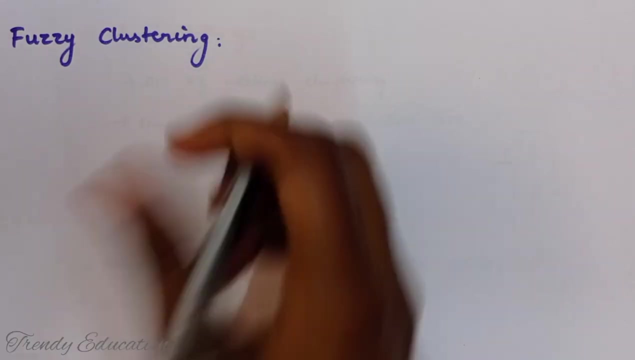 Now fuzzy clustering. So what is fuzzy clustering? in a sense, Each and every object, that is, every object that belongs to each cluster, with a membership weight. Here we are having something called a membership weight. So this is the term, which is different from others. 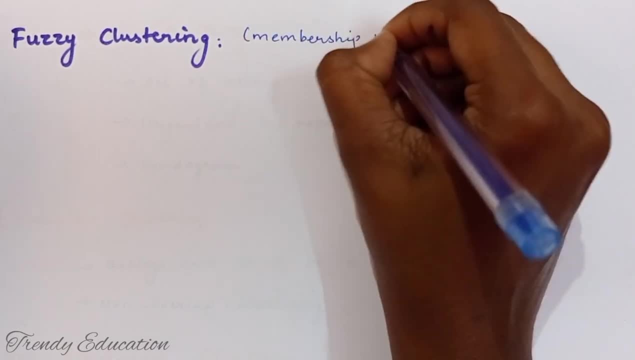 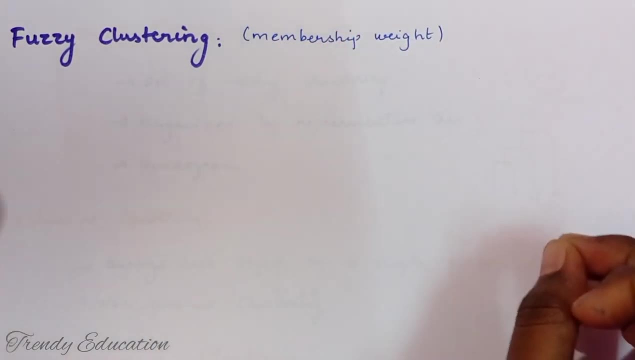 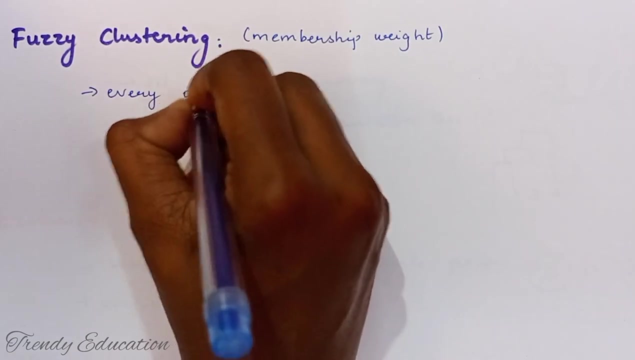 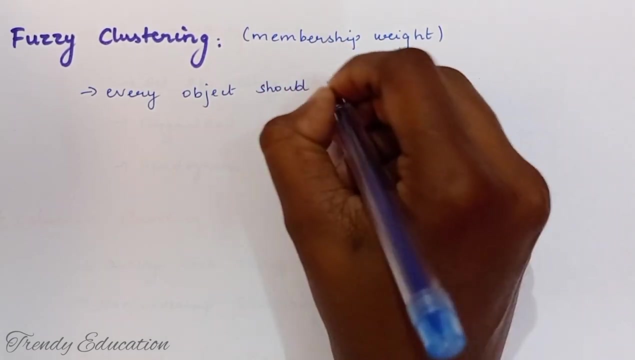 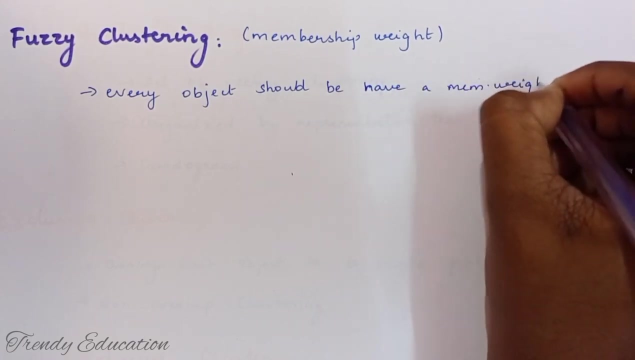 What it is is membership weight. If the objects that is added as membership weight is Between 0 and 1, it is clustered as fuzzy clusters. Every object, that is, every object within this cluster, should be Have a membership weight Between 0 and 1.. 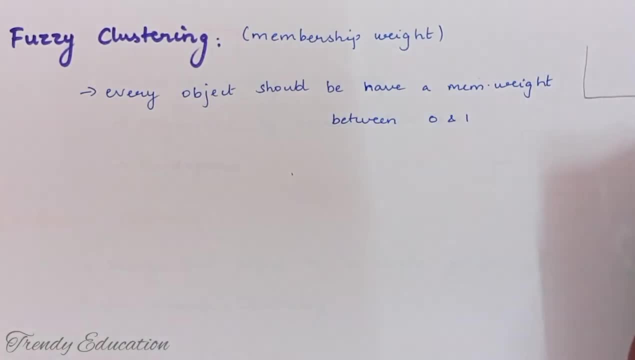 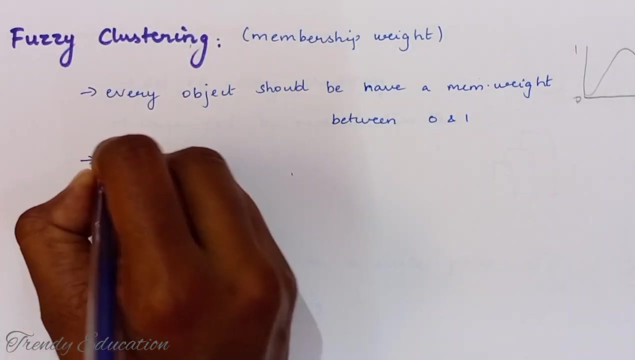 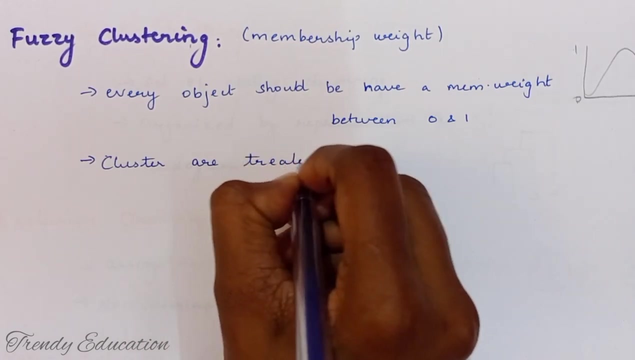 That is, The membership weight is measured. if, If the objects membership weight is between this 0 and 1, then it is clustered as a fuzzy clustering And here the sets are treated as fuzzy sets, that is the cluster, Or treated as like the fuzzy sets. 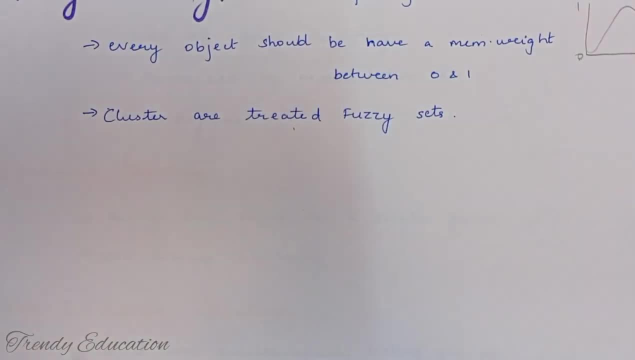 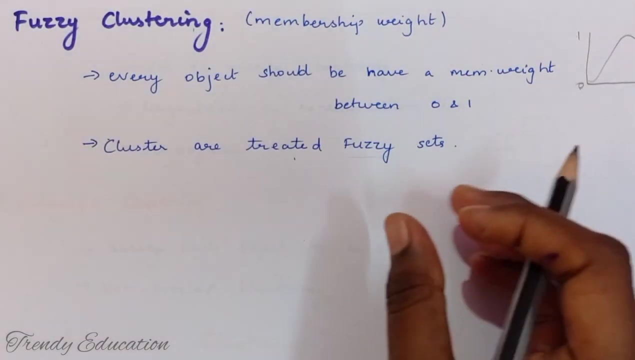 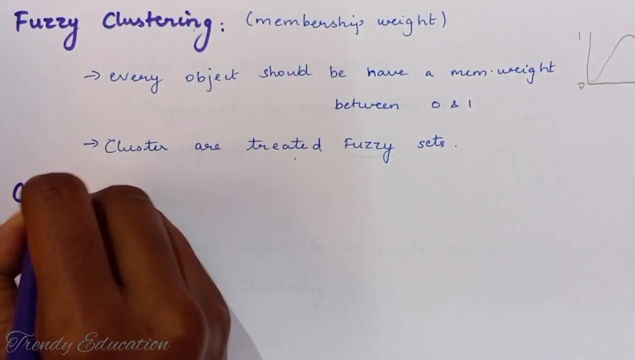 And if you want to know what is Fuzzy is like it's not determined. it's not clearly determined like we can assume people as poor, very poor, high, very high like this we are. we could not be able to determine what type it is actually. so this is what fuzzy, yeah, now coming to the complete clustering, 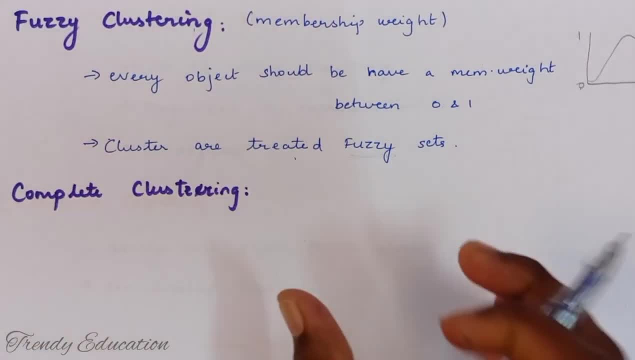 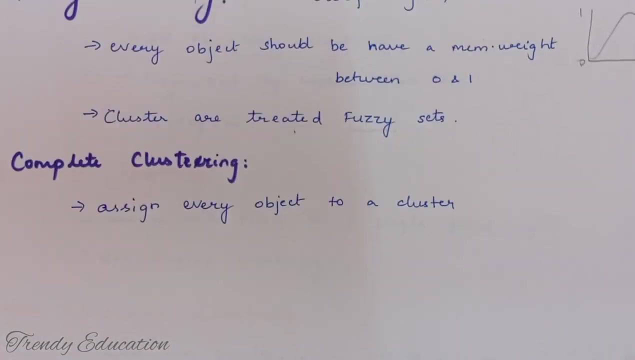 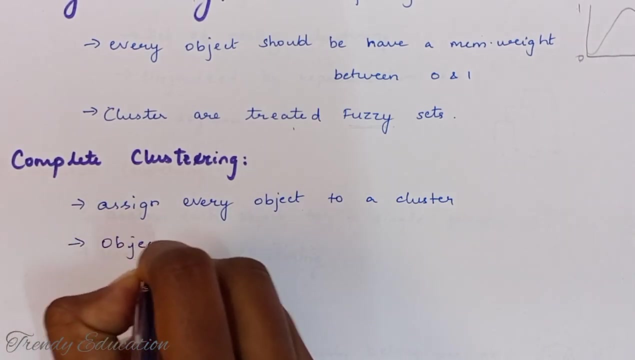 So what is complete clustering? in the sense each, every object, each and every object in the Dataset will have a cluster, every object in the data set will have a cluster. so this is what complete. Here not even one data is left. so each and every data in the data set will be clustered to any of the cluster set. so this is what the complete and here the cluster is sorry, the object. here the object is very desired, desired object. 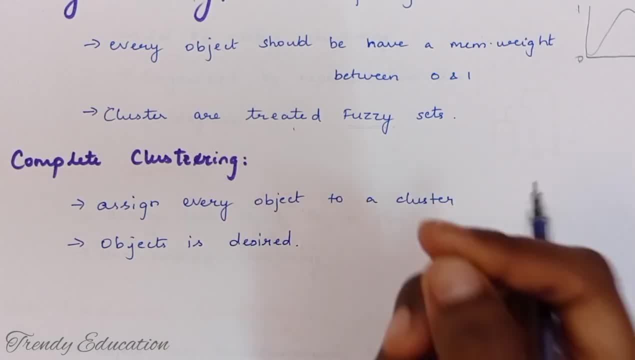 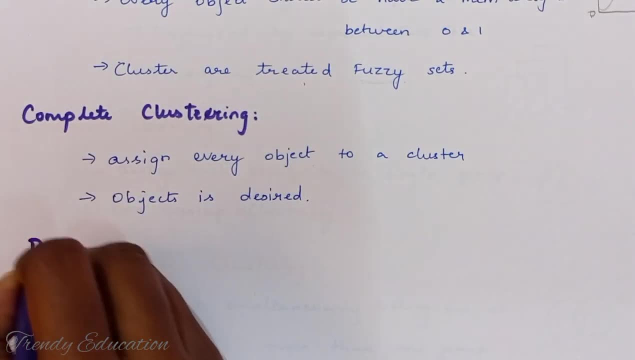 Because There is not even a single data which is left. so every object is desired. And now coming to the last type, which is the partial clustering. So the partial clustering is exactly opposite of the complete clustering. here there are some data which might be left. 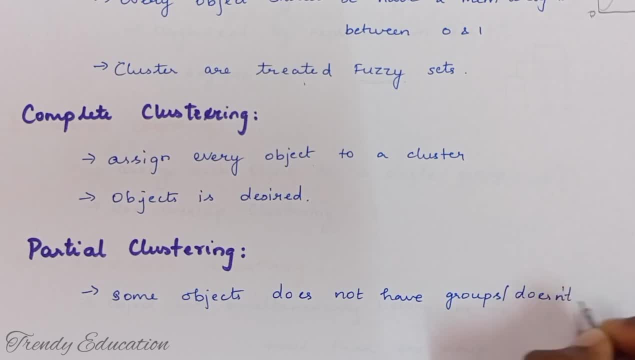 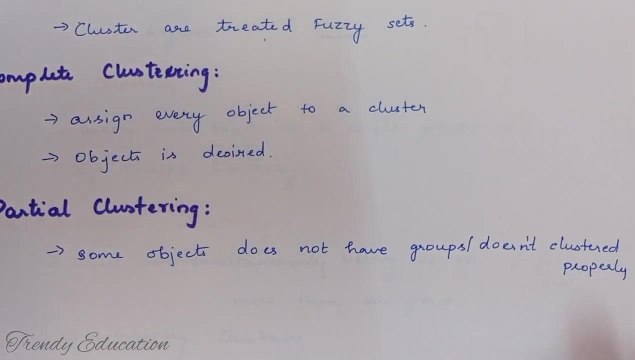 Or doesn't Clustered properly. So what is the reason? the is there might be a background noise or there might be a error data. so this is the main reason for this partial clustering. and it doesn't Have desired object because there are some left objects. 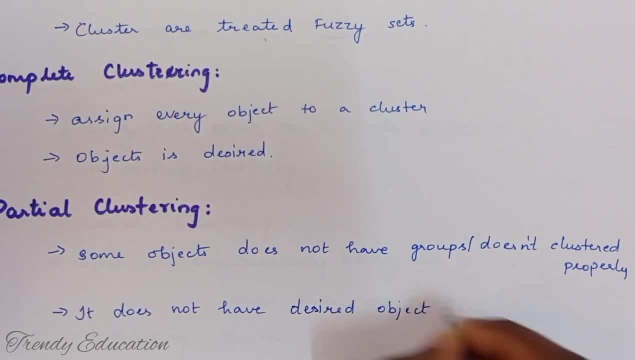 So, And yeah, this is what the types of clustering. if you have any, If you have any doubts, then ask me in the comments and also, if you want me to explain any type of video in computer science, you can directly ask me the command section. and yeah, thank you, bye.